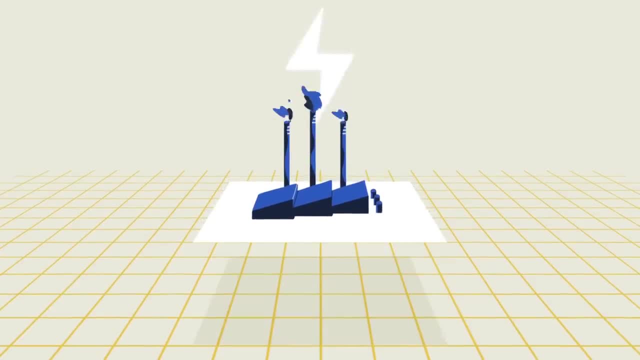 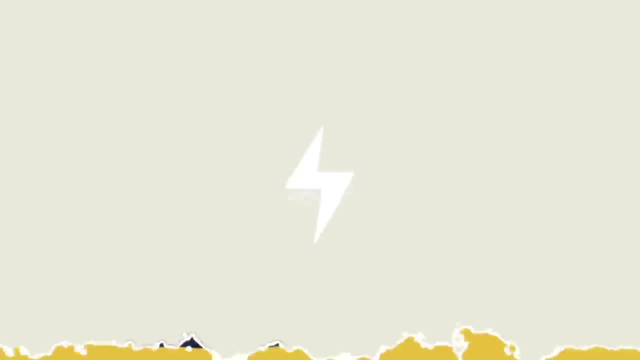 For each power source, there's variability in how much power it can generate per square meter, but these numbers give us a general sense of the space needed. Of course, building energy infrastructure in a desert, a rainforest, a town or even in the ocean are completely different prospects. 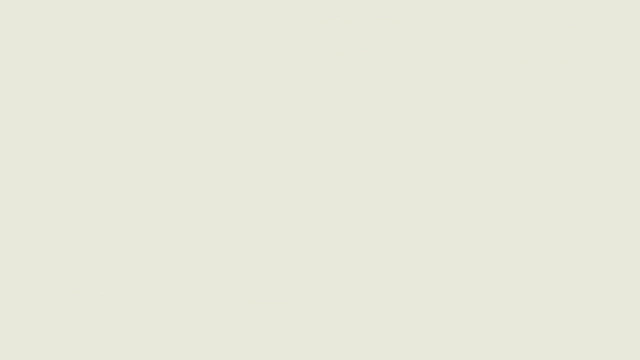 And energy sources monopolize the space they occupy to very different extents. Take wind power. Wind turbines need to be spread out, sometimes half a kilometer apart, so that the turbulence from one turbine doesn't reduce the efficiency of the others. So much of the land needed to generate wind power. 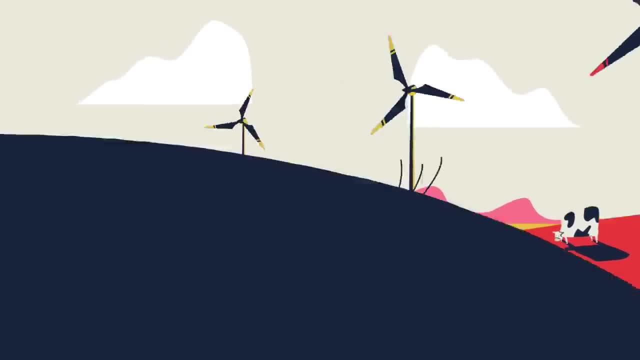 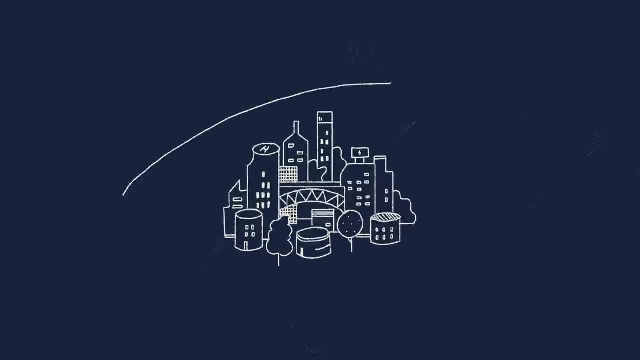 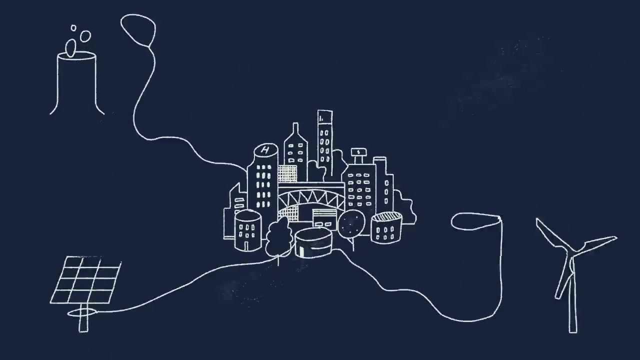 is still available for other uses, But the baseline amount of space still matters because cities and other densely populated areas have high electricity demands and space near them is often limited. Our current power infrastructure works best when electricity is generated where and when it's needed. 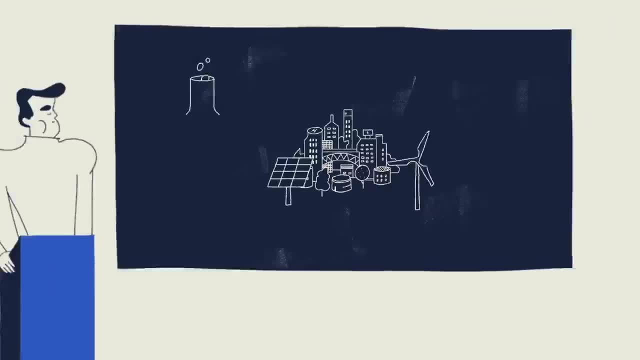 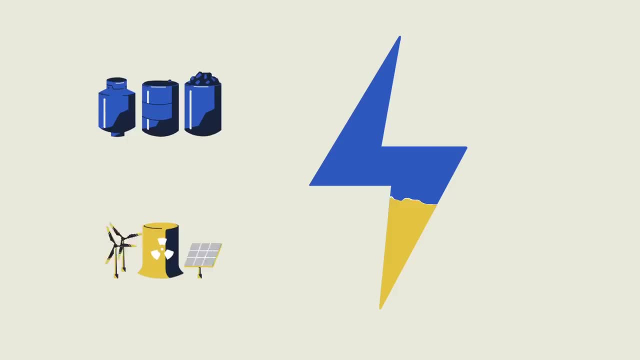 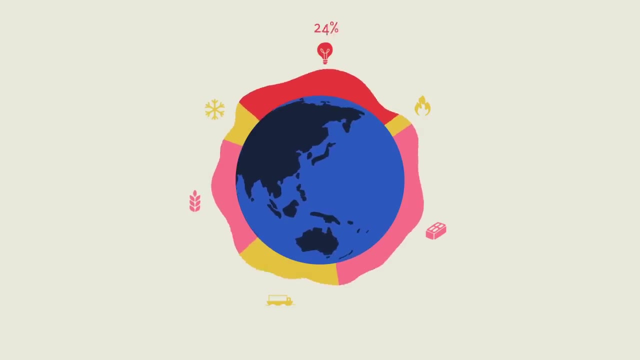 rather than being stored or sent across long distances. Still, space demands are only part of the equation. As of 2020, two-thirds of our electricity comes from fossil fuels. Every year, electricity generation is responsible for about 27% of the more than 50 billion tons of greenhouse gases we add to the atmosphere. 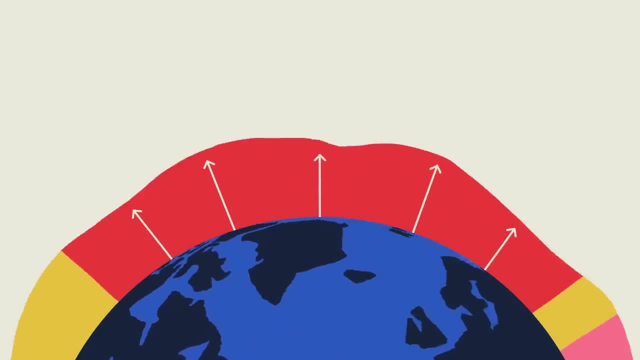 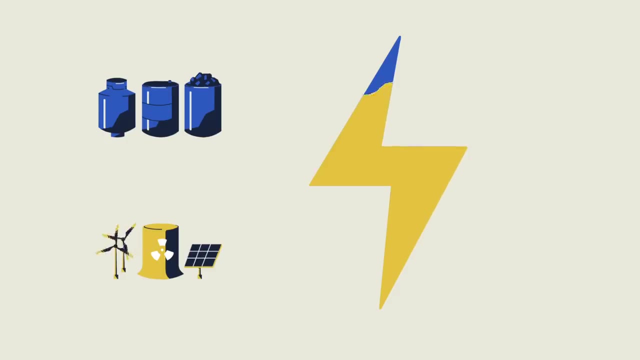 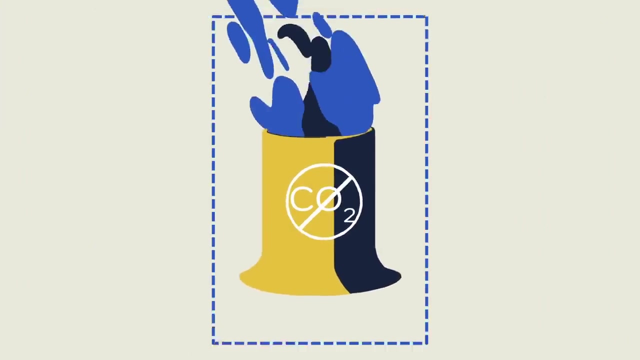 accelerating climate change and all its harms. So although fossil fuels require the least space of our existing technologies, we can't continue to rely on them. Cost is another consideration. Nuclear plants don't emit greenhouse gases and don't require much space, but they're way more expensive to build than solar panels or wind turbines. 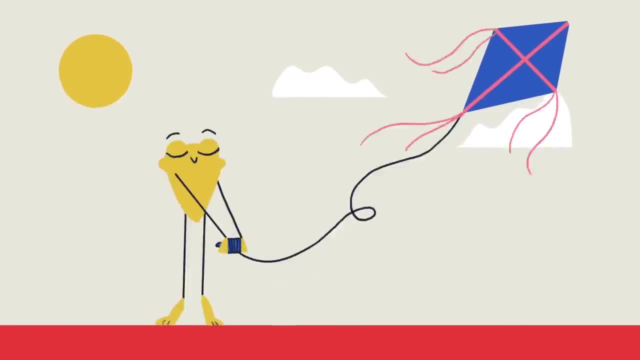 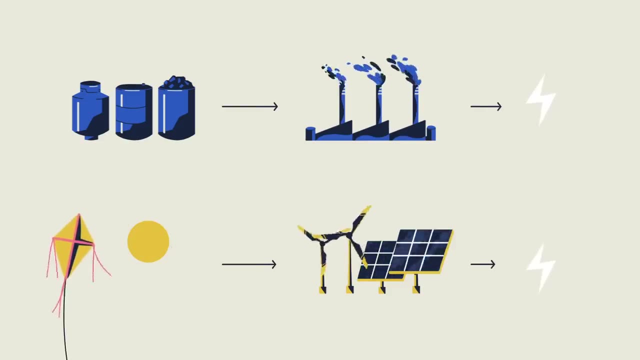 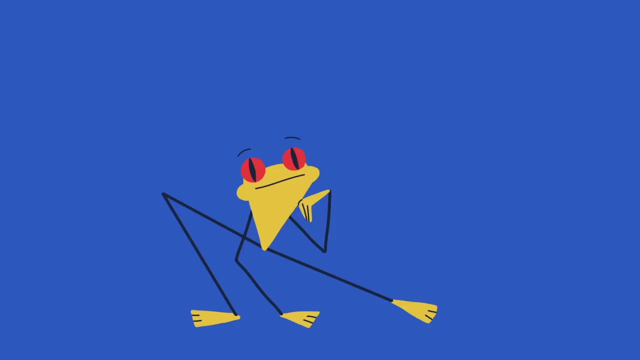 and have waste to deal with. Renewables have almost no marginal costs, Unlike with plants powered by fossil fuels, you don't need to keep purchasing fuel to generate electricity, But you do need lots of wind and sunlight, which are more available in some places than others. 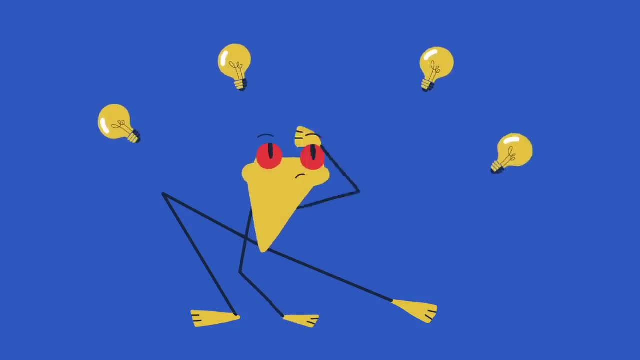 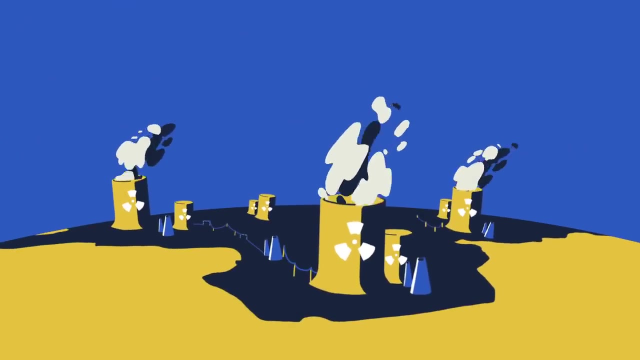 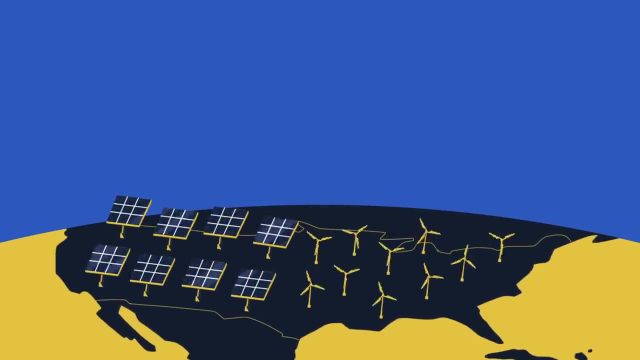 No single approach will be the best option to power the entire world while eliminating harmful greenhouse gas emissions. For some places, nuclear power might be the best option for replacing fossil fuels. Others, like the US, have the natural resources to get most or all of their electricity from renewables. 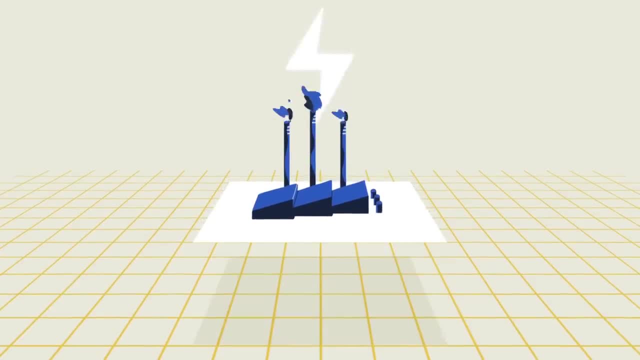 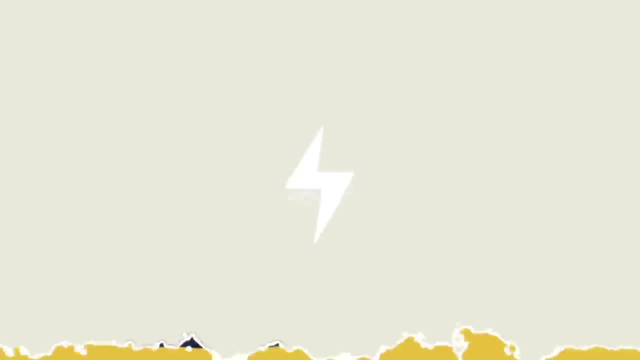 For each power source, there's variability in how much power it can generate per square meter, but these numbers give us a general sense of the space needed. Of course, building energy infrastructure in a desert, a rainforest, a town or even in the ocean are completely different prospects. 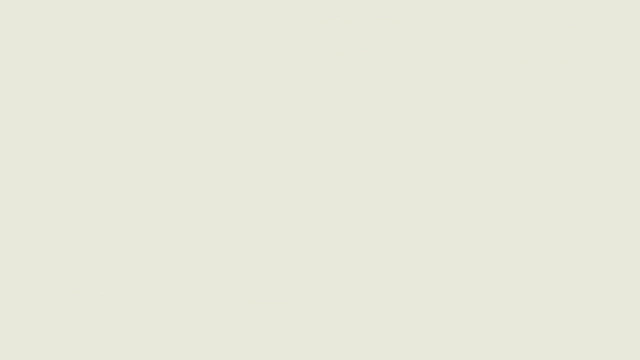 And energy sources monopolize the space they occupy to very different extents. Take wind power. Wind turbines need to be spread out, sometimes half a kilometer apart, so that the turbulence from one turbine doesn't reduce the efficiency of the others. So much of the land needed to generate wind power. 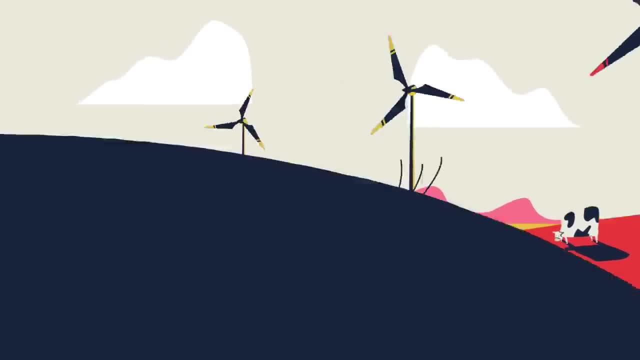 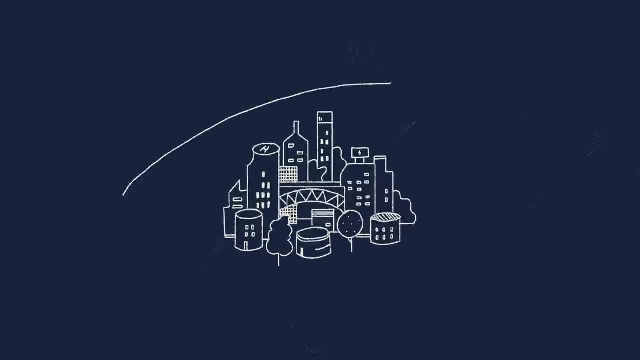 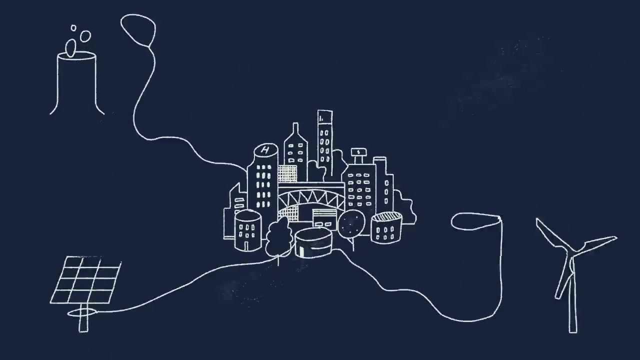 is still available for other uses, But the baseline amount of space still matters because cities and other densely populated areas have high electricity demands and space near them is often limited. Our current power infrastructure works best when electricity is generated where and when it's needed. 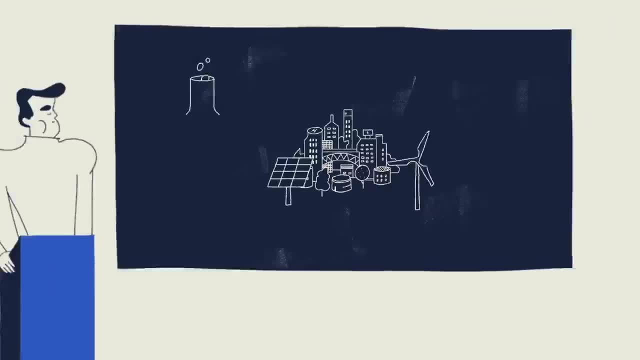 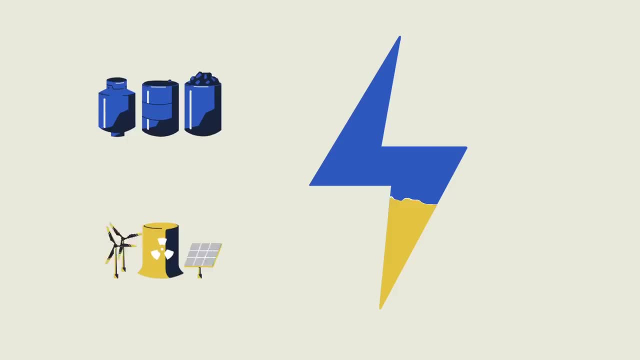 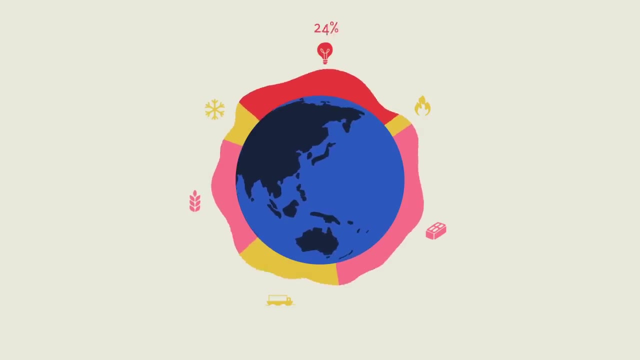 rather than being stored or sent across long distances. Still, space demands are only part of the equation. As of 2020, two-thirds of our electricity comes from fossil fuels. Every year, electricity generation is responsible for about 27% of the more than 50 billion tons of greenhouse gases we add to the atmosphere. 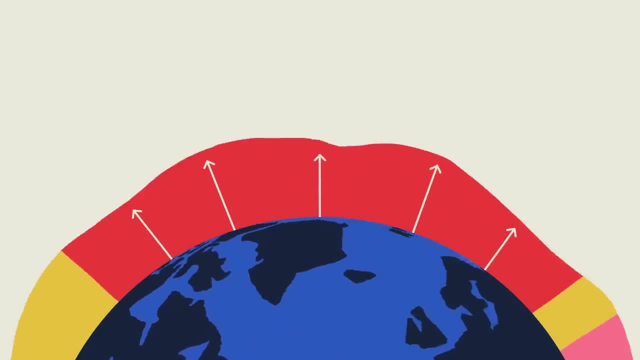 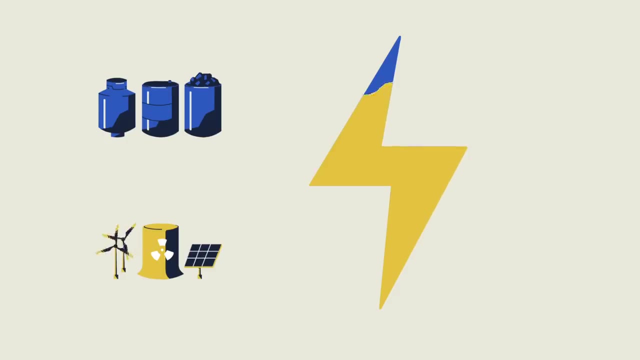 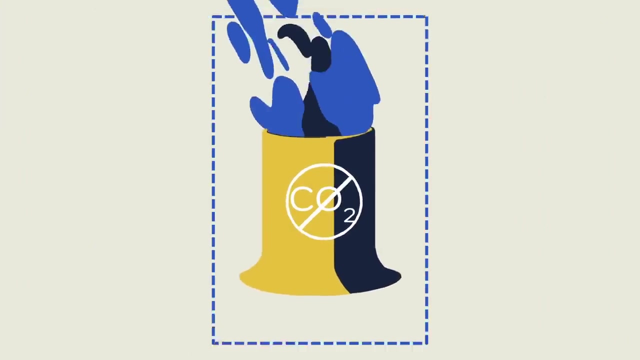 accelerating climate change and all its harms. So although fossil fuels require the least space of our existing technologies, we can't continue to rely on them. Cost is another consideration. Nuclear plants don't emit greenhouse gases and don't require much space, but they're way more expensive to build than solar panels or wind turbines. 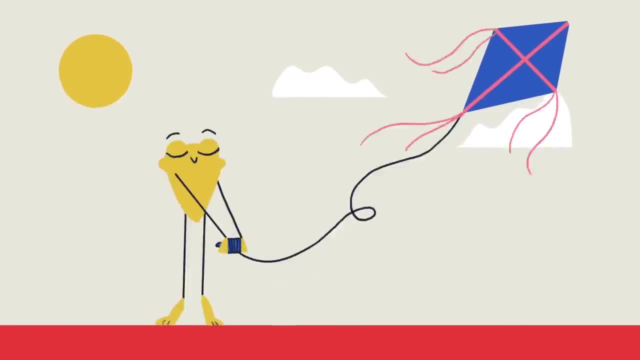 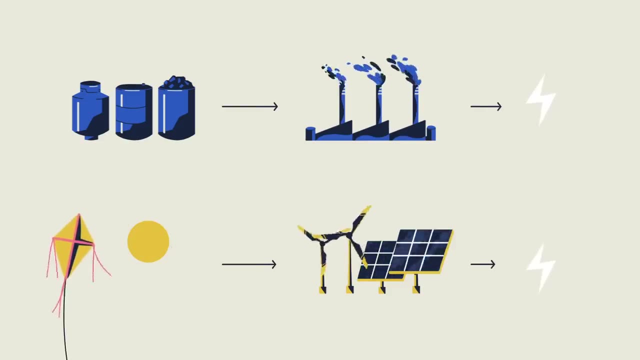 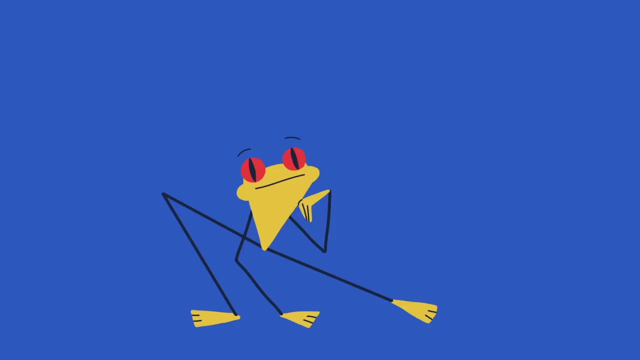 and have waste to deal with. Renewables have almost no marginal costs, Unlike with plants powered by fossil fuels, you don't need to keep purchasing fuel to generate electricity, But you do need lots of wind and sunlight, which are more available in some places than others. 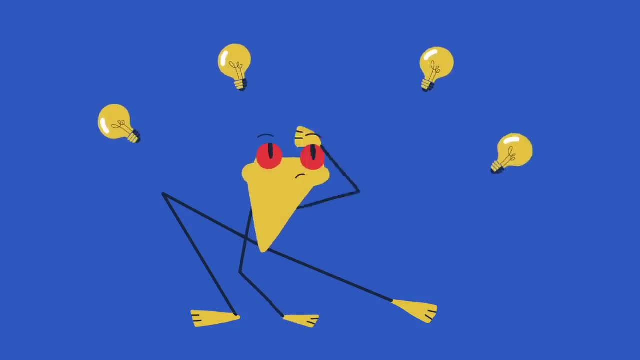 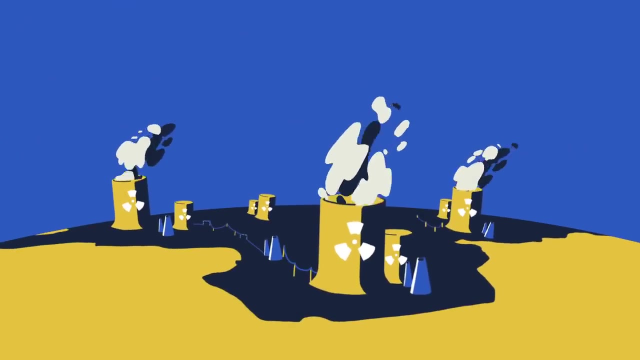 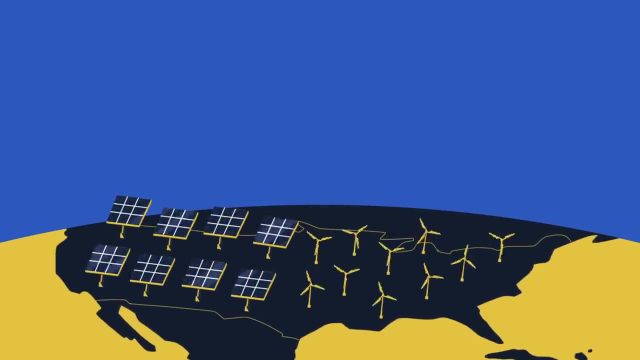 No single approach will be the best option to power the entire world while eliminating harmful greenhouse gas emissions. For some places, nuclear power might be the best option for replacing fossil fuels. Others, like the US, have the natural resources to get most or all of their electricity from renewables. 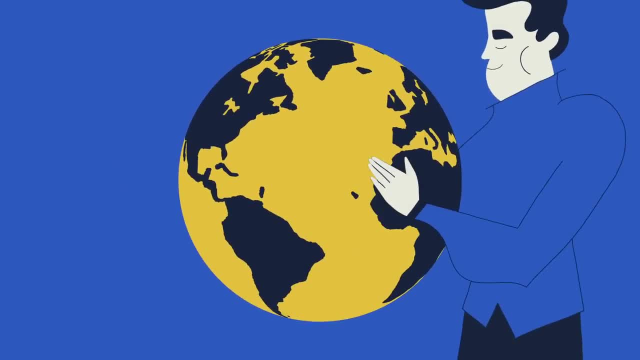 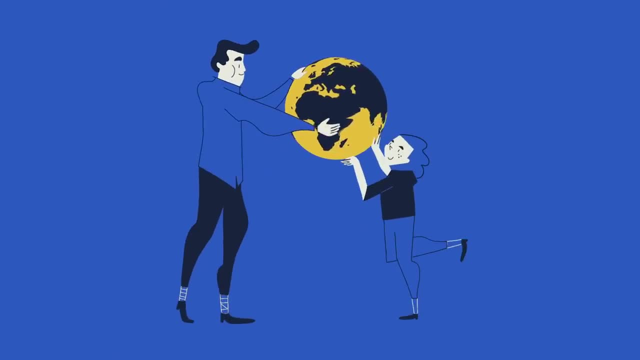 And across the board, we should be working to make our power sources better: safer, in the case of nuclear, and easier to store and transport, in the case of renewables. OK, so that's how much space we need to power the world, But exactly how much electricity do we need? 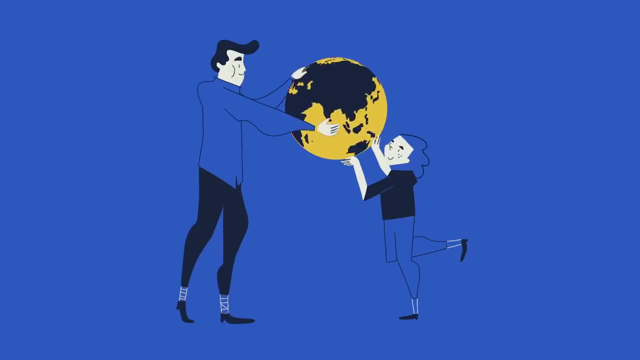 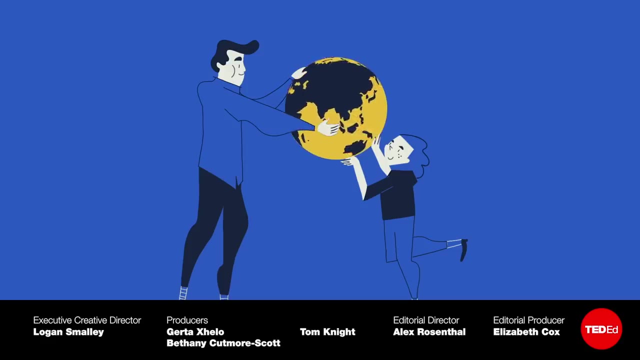 Find out with this video, Or watch this video to learn, how boring old cement might just be a superhero in disguise, ready to save the world. 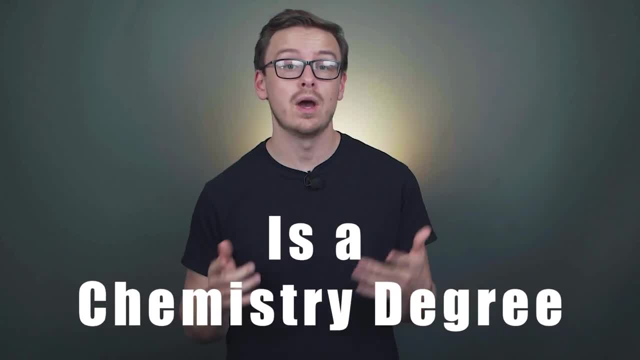 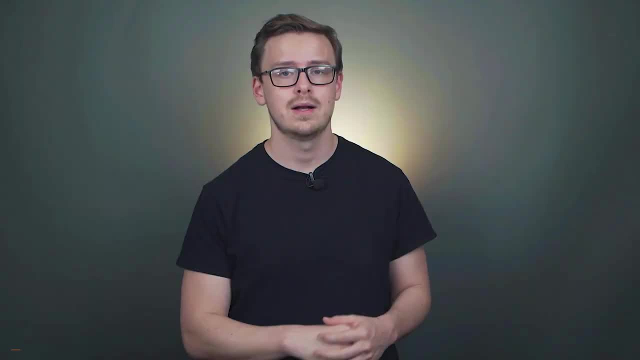 Is studying a chemistry major to get a chemistry degree worth it. That's what we're going to be talking about today, but before we get into that, make sure to gently tap the like button in order to defeat the evil YouTube algorithm. On this channel, we talk about personal finance, college. 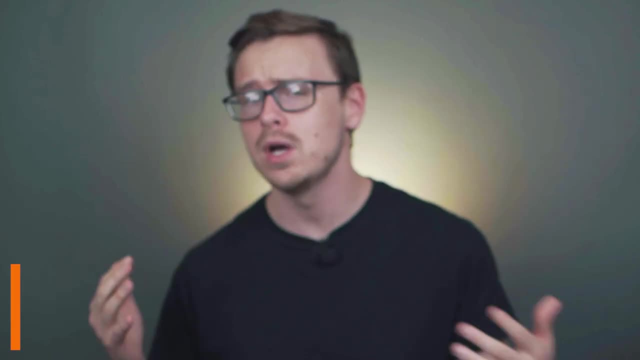 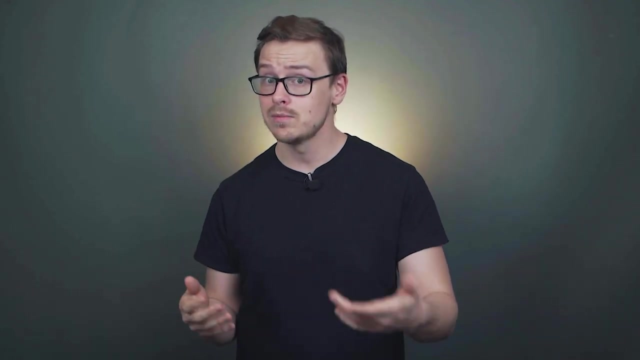 degrees, careers and opportunities that are going to lead you to success, and we also go over how you can avoid some of the common financial traps that so many people end up falling for. If that sounds like something that interests you and you haven't done it already, go ahead and hit that. 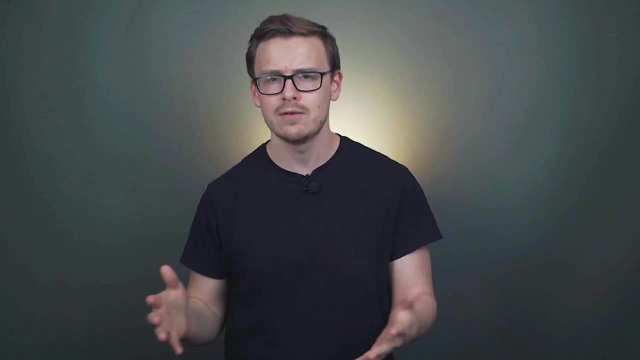 subscribe button and ring the notification bell, Only like 18% of you have, so that you never miss an opportunity. But let's jump into it. Back to the main subject. Is a chemistry degree worth it? We're going to be talking about this today, but first let's go ahead and define what a chemistry 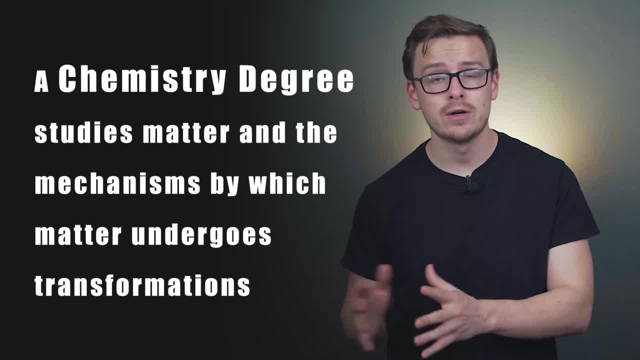 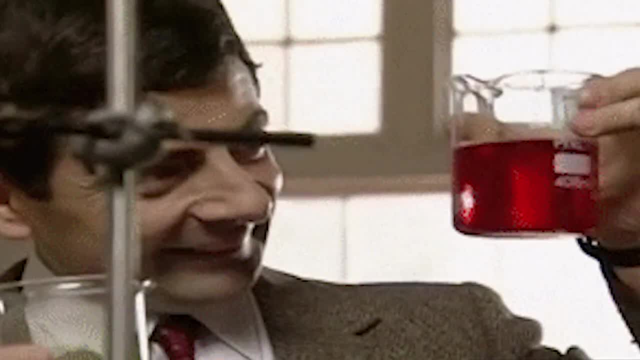 degree is. So a chemistry degree is going to be the study of matter and all of its different forms and how it transforms between one form or the other. There's a lot of science, of course, but you're also going to be doing lab work as well as mathematics. There's about 14,000 people that 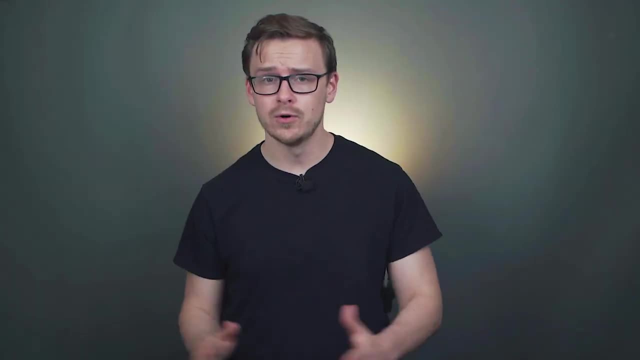 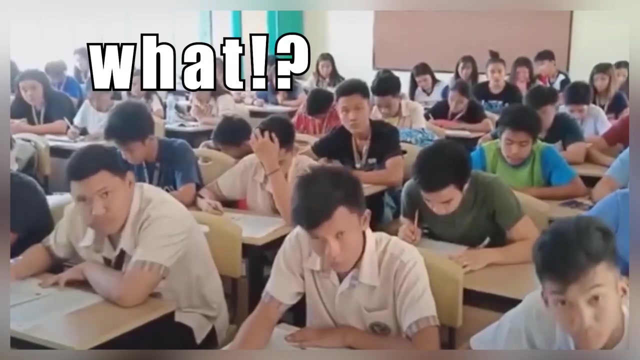 graduate with a bachelor's in chemistry every year. Now I've said this before in a lot of other videos, but I have to say in this one as well: science degrees compared to the other STEM degrees in my opinion are a little bit overrated A lot. 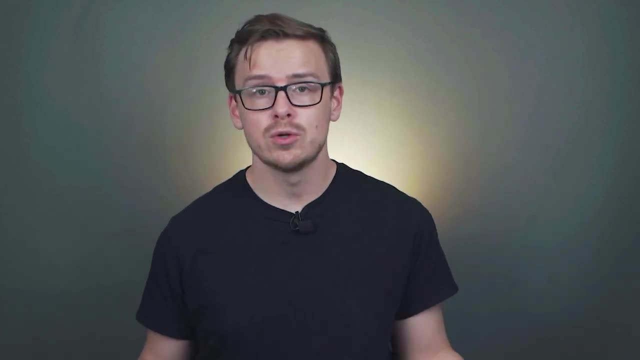 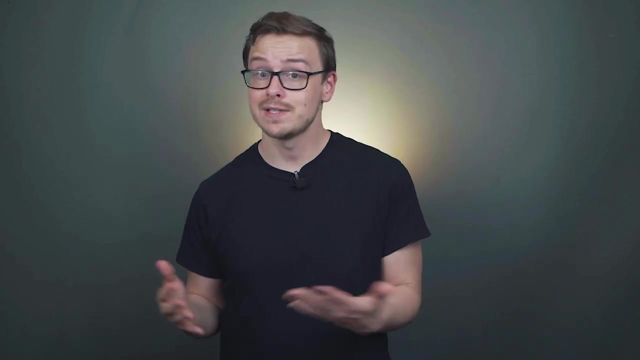 of people think that STEM degrees are amazing and if you get any type of STEM degree, companies are just going to be lined up ready to give you a job right after you graduate. and that's just not true. The truth is, if you get some science bachelor's degrees and you expect to get a job, chances are. go on average about $40,000 a year. you're going to have to get a master's or a doctorate, And if in debt in order to get your degree, you can't just snap your fingers and make it go away. Now we're going to go over four different sections here. The first one is going to be: 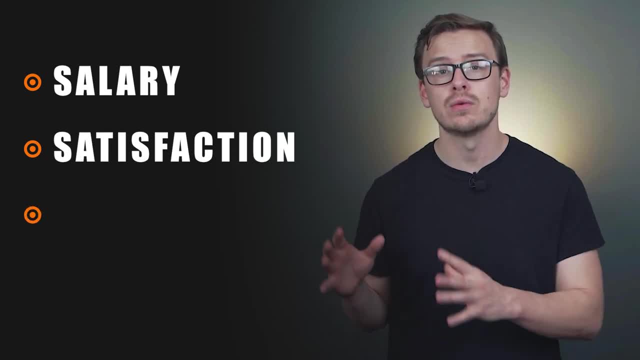 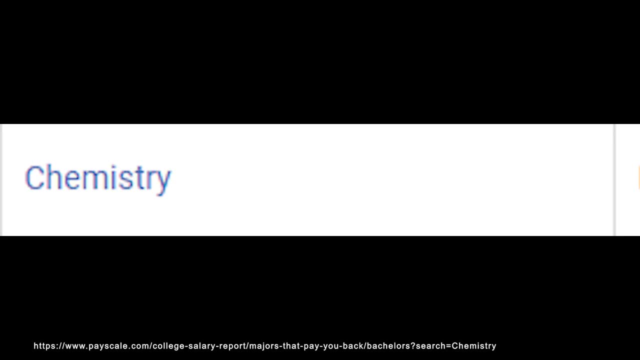 salary. Then we're going to talk about satisfaction, Then we're going to go over demand And then, lastly, we're going to talk about X factors. First, let's go ahead and talk about salary. With a chemistry degree, you would expect to make around $49,000 a year in your first five years working and then mid-career pay would be $93,000.. You can compare this to petroleum engineering, which is an extremely high-paying degree, Or recreational therapy, which doesn't pay very well, And you're going to see that it is somewhere.